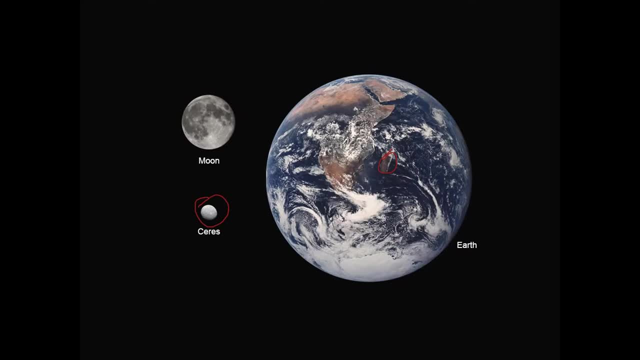 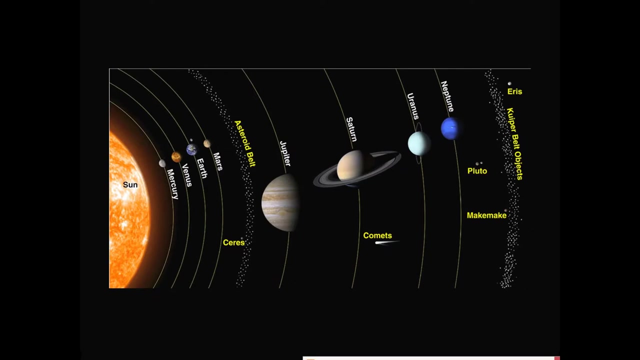 this. The point is that it's full of a lot of small asteroids. They're actually small rocks. It's usually metal. In the future you could go there and mine them. There's probably all kinds of interesting minerals in them. They. 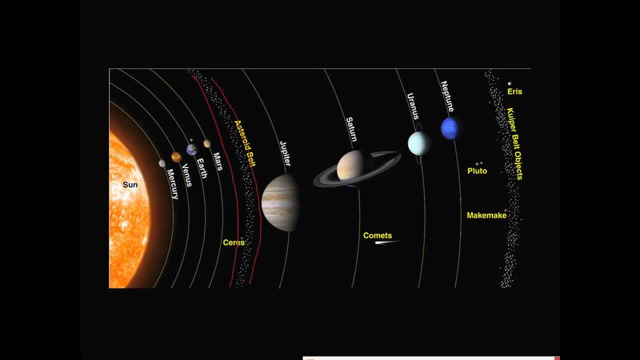 are in this area, here the asteroids. Then there's a huge field outside Pluto. It's called the Kuiper belt. Actually, right now there is one satellite going out there. It went past Pluto last year, I think. No, it was actually this year. Then it is out in the Kuiper belt now. Then for 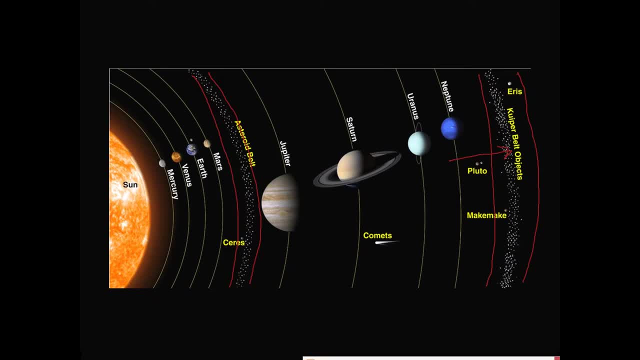 the first time ever we can get a better close-up. look at that. There has been earlier satellites going out there, but they were built in the 1970s or so. They're not really able to transmit pictures and stuff. This one, this satellite, was put up in 2006 and had sort. 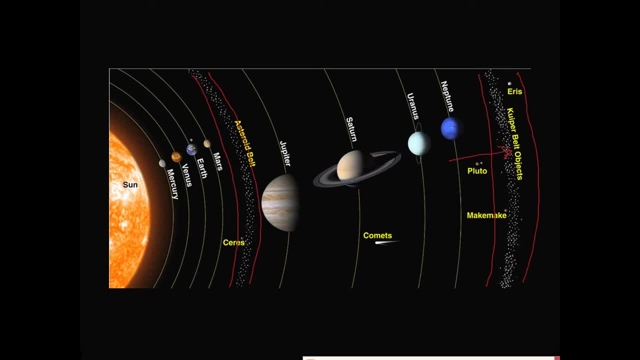 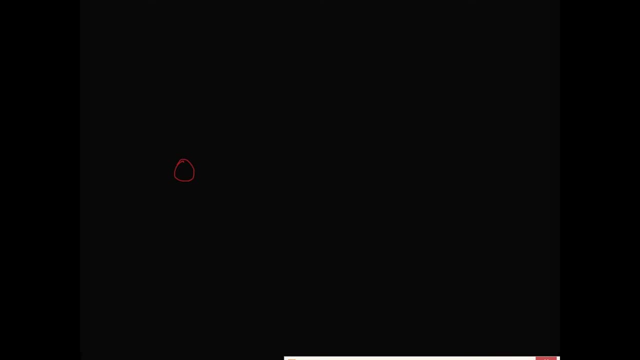 of pretty modern cameras. It has traveled more than 4 billion kilometers by now. If we have the sun here, then the planets have kind of nice orbits around the sun. Then we have some small rocks That has very elliptical orbits. They are called comets. Then they return every 70 years. or so, or every 200 years and so on. They have a very, very long distance to go around the sun with. Their years are a lot. What I mean by that is that Earth takes one year to go around the sun and some of them take 70 or 200 or something years to. 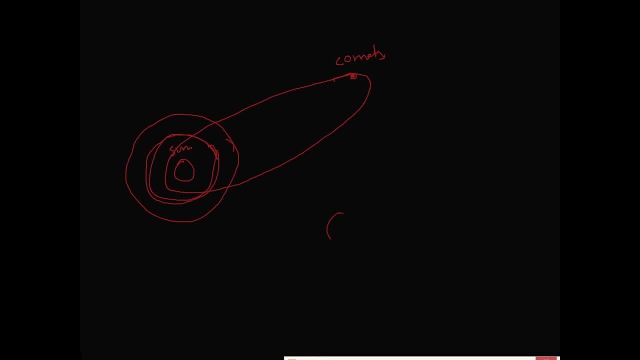 go around the sun. They are usually. they have an ice core. Then when they come close to the sun, then it starts to evaporate. These comets, it looks like they have a tail on the sky. This is a characteristic of a comet. 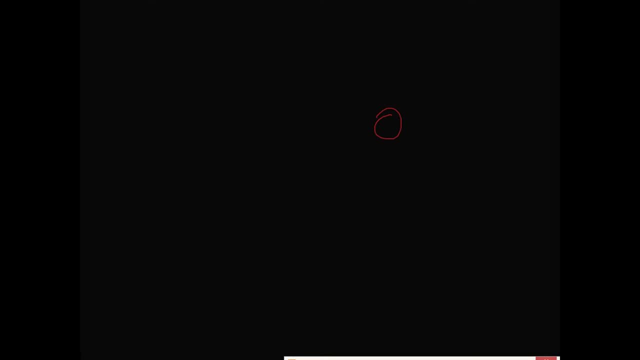 Asteroid. It is just a rock, but it has a sort of normal orbit around. if we have the sun here, It's just traveling around this way. Once in a while we have Earth here. Once in a while a little debris come down here to Earth's atmosphere and it starts to burn up. This 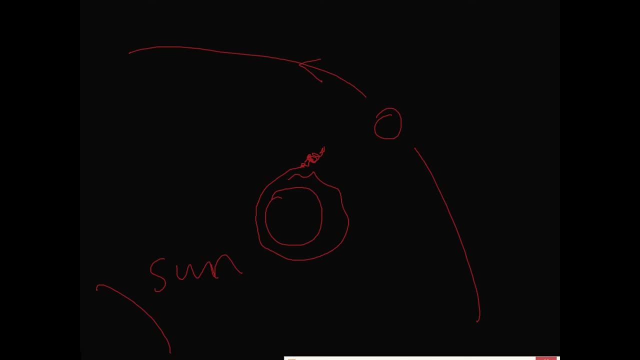 is called a falling star, a shooting star. It is also called a meteor. When the meteor is burning up, it's usually burning up because it's very rare that they actually land on Earth. If they make it down to Earth without burning up, you call the. 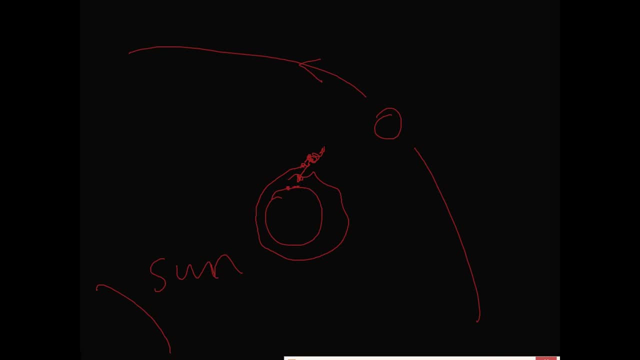 small debris somewhere down. I will just paint it in yellow here. This little debris is called a meteorite Here. meteorite That's the debris on Earth. The meteor is on the sky with a tail. It's burning Out here before it actually comes into the atmosphere. it's also called a meteoroid. 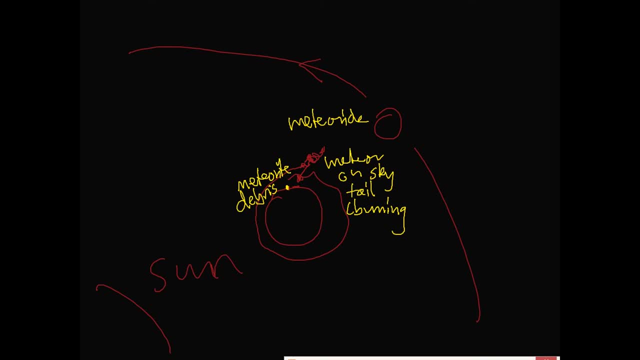 Meteoroid, Meteoroid, Meteoroid. It's coming out in the atmosphere. It can be in the Universe and out here, an asteroid. Actually, all of these names it's actually the same stuff: Smaller rocks. They can be in the lane out. here They are called an asteroid. 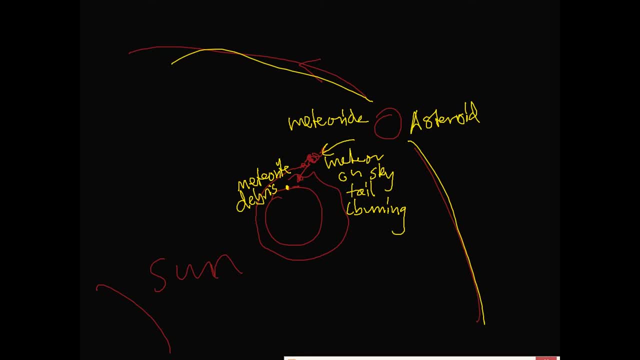 They can be coming here, called a meteorite. They burn up in the atmosphere. it's a meteor, Then the rock that you can pick up on Earth rarely is a meteorite. Meteoroid with a T- These are the names of these stellar things. 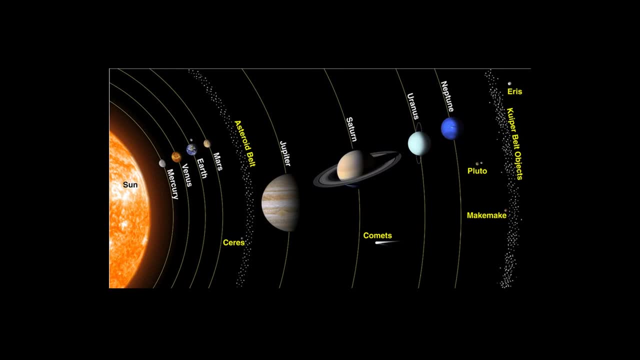 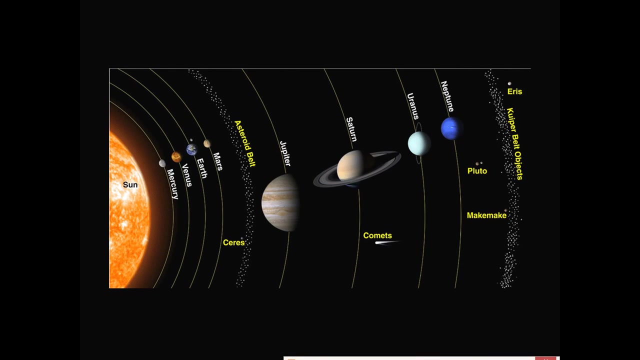 Going back to a picture that's a bit nicer than my picture. there's also the subject of dwarf planets. These are very big asteroids. Some people say that Ceres is a small. We have Ceres here and then we have, for example, Pluto.